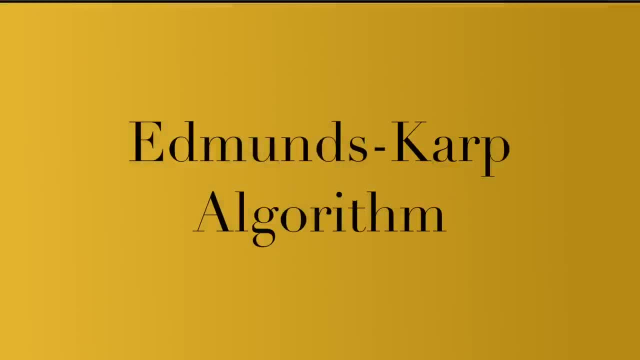 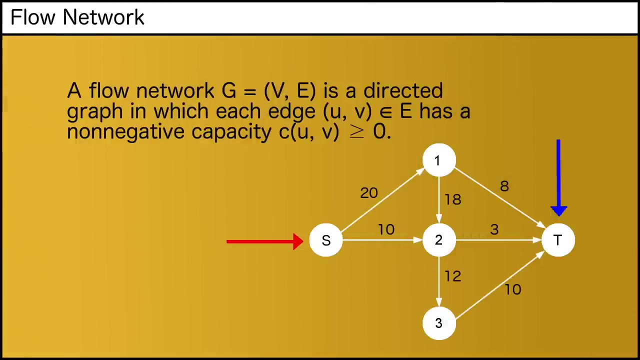 Hi guys, I'm Ben and I'm Owain, and we're going to be talking about the Edmonds-Karp algorithm. The Edmonds-Karp algorithm finds the max flow on a flow network. But what is a flow network? Well, Owain, a graph with no's and directed edges with capacity can. 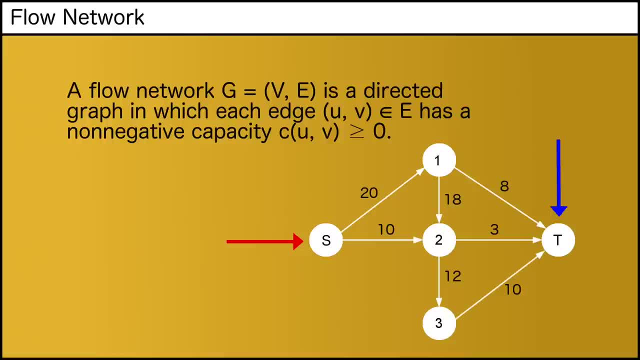 be interpreted as a flow network, metaphor being the flow of water through pipes. We distinguish two vertices in a flow network: the source being the origin of the flow, shown with the red arrow, and the sink being where the flow terminates, shown by the blue. The. 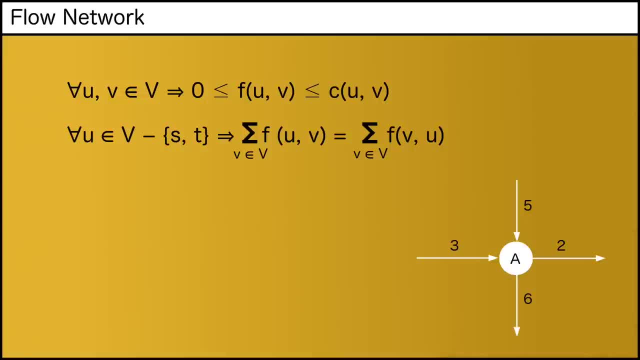 first line formalises the fact that a flow along an edge is going to be greater than or equal to zero, but not more than that edge's maximum capacity. The second line means that for all nodes except for the source and the sink, the flow is conserved. This means that 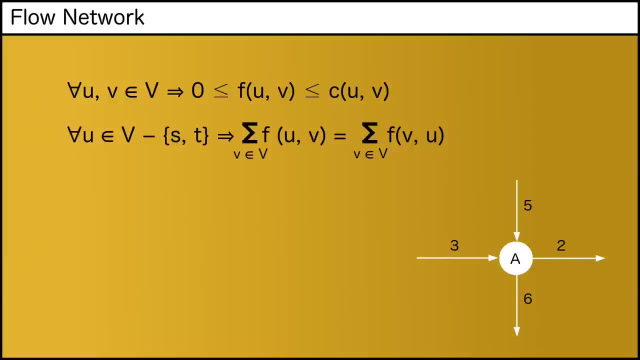 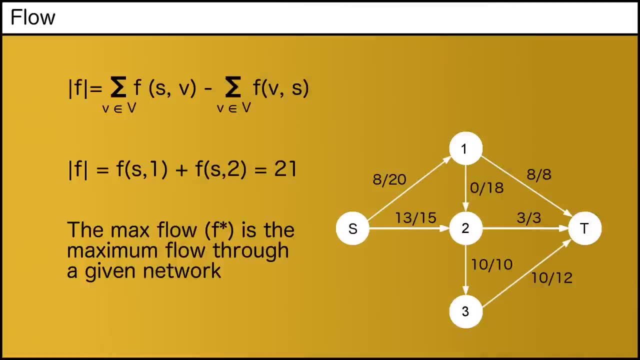 all the flow that enters the node must leave it. For example, eight enters. The flow through a network is the amount of flow leaving a source minus the amount flowing into the source. However, we won't include any flow going into the source In this case. 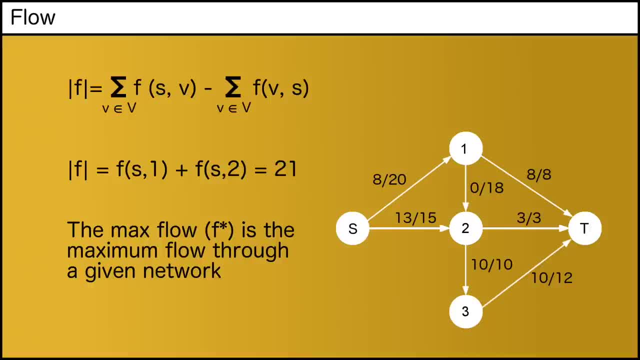 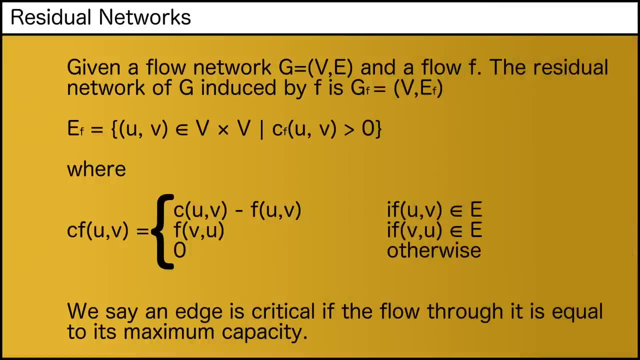 8 and 13 leave the source, which gives a flow of 21.. The max flow is the maximum possible flow through a given network. When you have a flow network and a flow, you can work out the residual network which shows additional available capacity. And this is how we 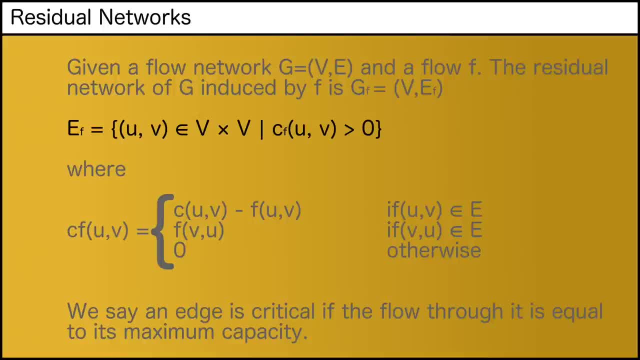 derive that This line describes how we get the edges on the residual network. It is done by only calculating the residual capacity for the every pair of vertical vertices on the flow network. The three possibilities we can encounter when calculating the residual capacity: CF. In the first case, it is additional flow that can be pushed along an edge which. 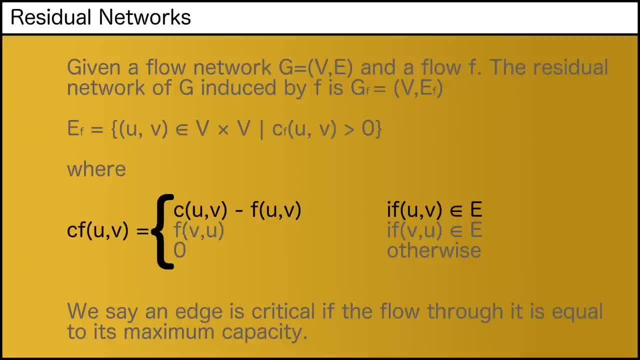 is given by that edge's maximum capacity minus the flow that's already flowing along it. If this flow along an edge in a flow network, the residual network will have that edge, but in the reverse direction, because flow can be pushed back along that edge. 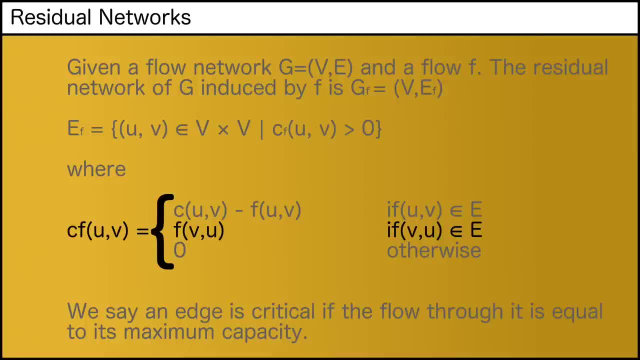 This gives the residual network the option to reduce the amount of flow along an edge. And if an edge doesn't exist between two vertices, there will be no edge on the residual network. We say an edge is critical if the flow through it is equal to its maximum capacity. 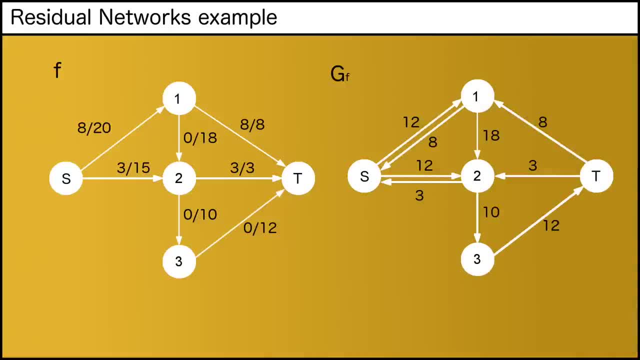 On the left we've got an example flow through a network and on the right is corresponding residual network. So if we take the edge between S and node 1 as an example, you can see that it is possible to push 12 more along the edge, because we are currently pushing 8 and its maximum capacity. 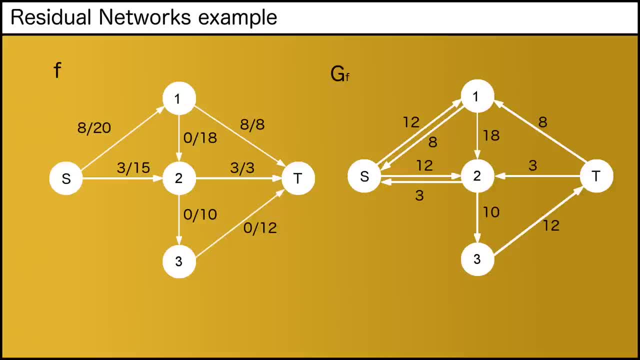 is 20.. So we can also push 8 back along the edge. This is what's indicated on the residual network. Now if we look at the edge between node 1 and the sink, we see that we can't push any more. 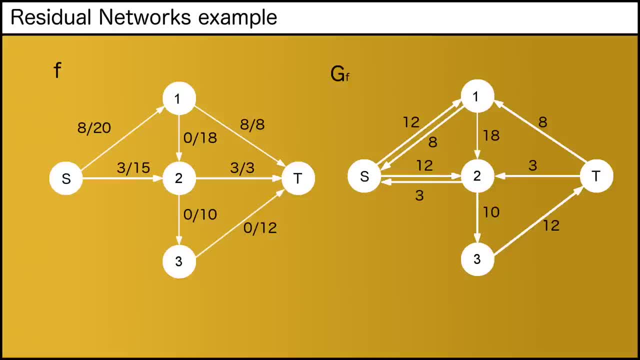 We can't push any more flow along this edge because it's at its maximum capacity. Therefore we call it a critical edge. So in the residual network it seems as if the edge is flipped because we can only push 8 back along that edge. 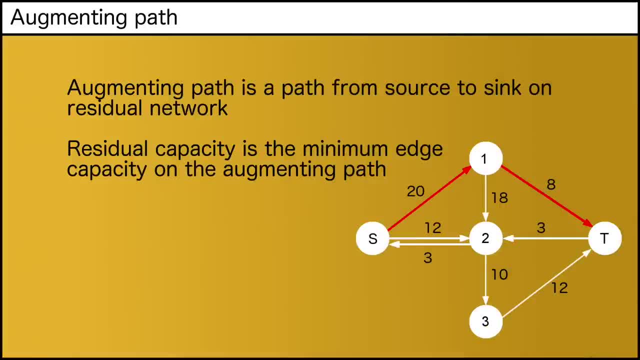 An augmenting path is simply a path from the source to the sink on the residual network. The residual capacity is the minimum edge on the augmenting path and this acts like a bottleneck to the flow along the augmenting path. An augmenting path can be added or augmented to a flow network. 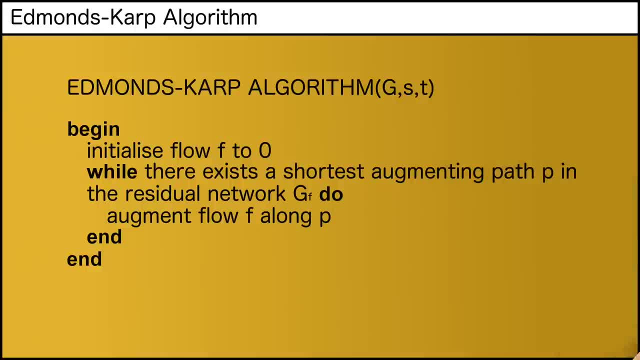 To increase the flow from the source to the sink. So here's the actual Edmunds-Karp algorithm that takes a graph and a source and a sink. It returns the max flow. It begins by initialising all the flow to be 0 and while there exists an augmenting 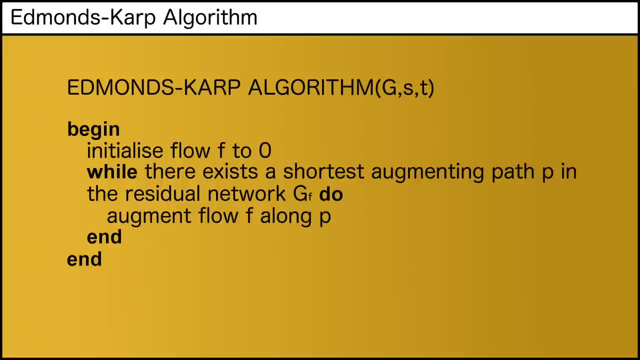 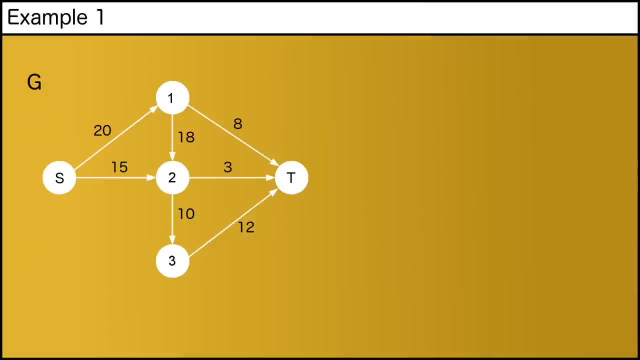 path in the residual network. that is a path from the source to the sink. you should find the shortest of these paths and add that flow onto the network. Here's an example of the Edmunds-Karp algorithm in action. Initially, the flow network is equal to its residual network. 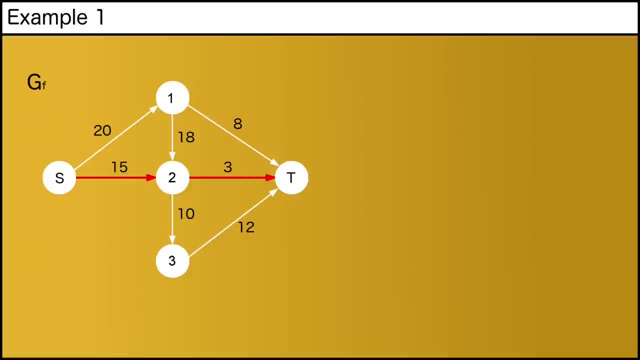 Because there's no flow going through the network. you can't push any back. So now we choose the shortest augmenting path on the network shown by the red arrows. This path has a residual capacity of 3.. So we can only push 3 out of the possible 15 along the edge between the source and node. 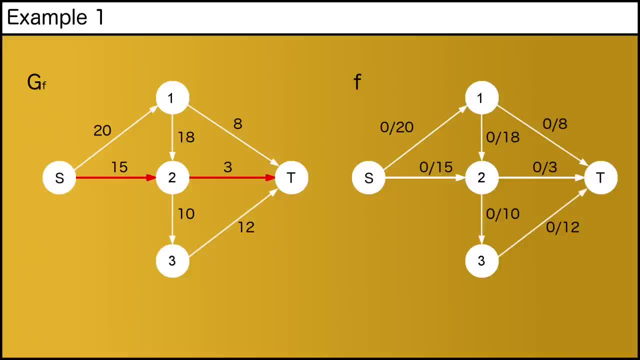 2. And we can push all 3 of the possible 3 between node 2 and the sink. We can now add this flow to the flow network. Now if you look at the updated residual network you can see it indicates the 12 additional. 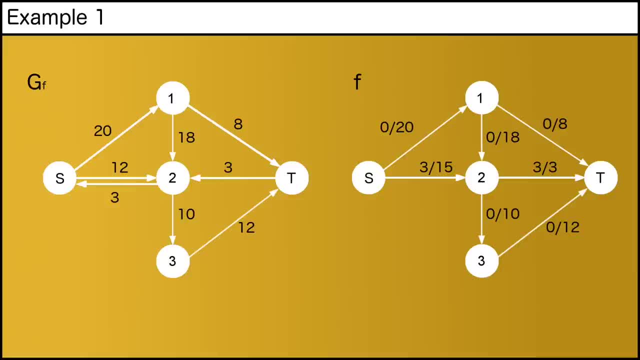 flow that can be pushed along the edge between S and node 2 and the 3 that can be pushed back along that edge. You can't push any more along the edge between node 2 and the sink because that edge was the critical edge, so you can only push 3 back. 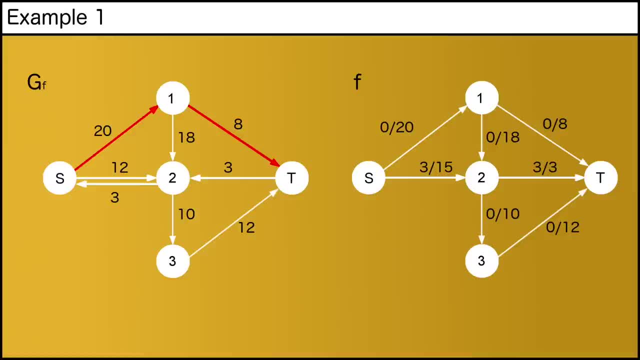 We now find the shortest augmenting path from the source to the sink on the new residual network. This new augmenting path indicated by the red arrows has a residual capacity of 8.. So on the edge between S and node 1, we can only push 8 of the possible 20 along that. 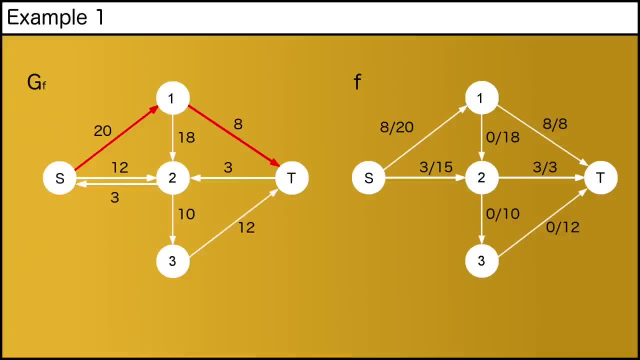 edge. We now add this flow of 8 to the network and update the residual network. Again, we find the shortest path from the source to the sink on the residual network And we can only push 10 along this path because that's the minimum of the 3 edges. 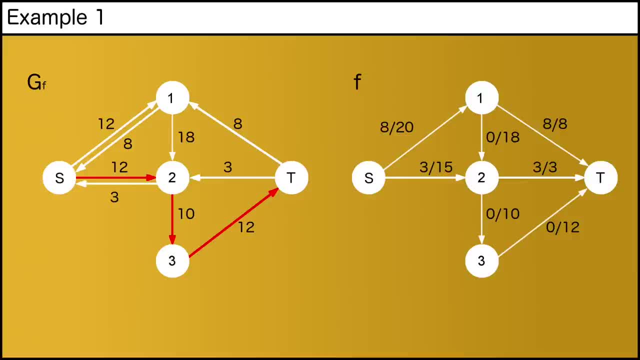 So, for example, If we take the edge between the source and node 2, we can push 10 out of the possible 12. This takes us up to a total of 13, because we were already pushing 3 and now we are pushing. 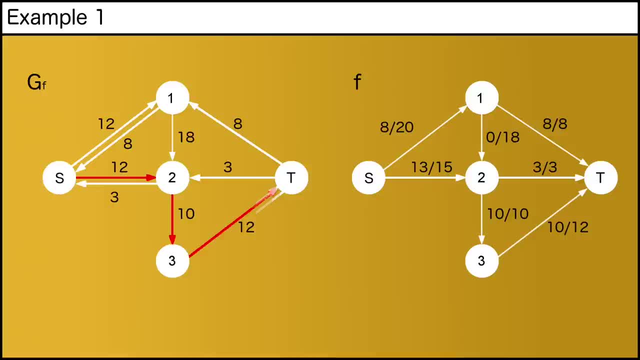 10 more. So, on the new residual network, we can either push that 13 back or push 2 more forward. Ben, would you like to try and find the next shortest augmenting path from the source to the sink? Yeah, why? 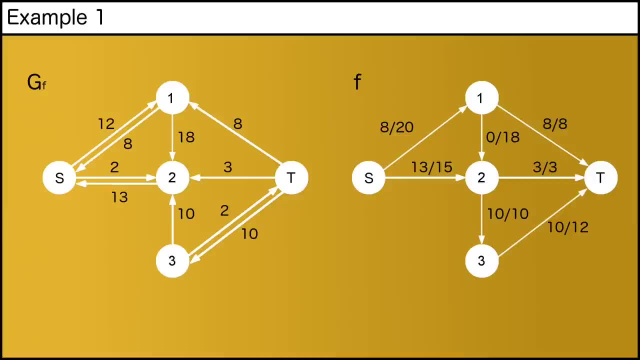 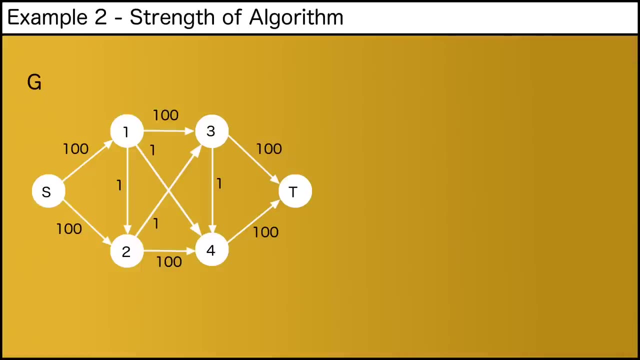 Oh wait, I can't. No, you can't Because there are no more. The algorithm is terminated. so the max flow is 21, because that's the total amount of flow leaving the source or entering the sink. Now we're going to show you the strength of the Edmonds-Karp algorithm. 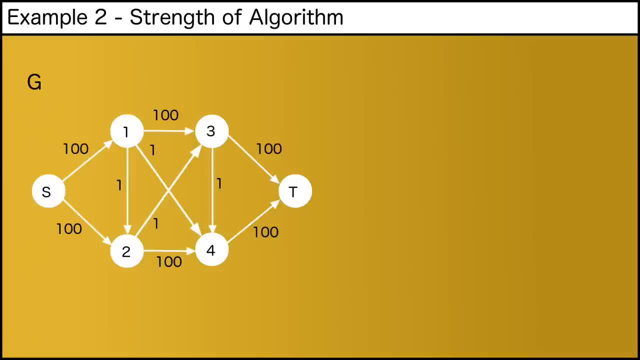 If we weren't to pick the shortest path for the augmenting path. every time an algorithm known as a Ford-Fulkerson- we may encounter a situation such as this: The augmenting path chosen could be a sub-optimal one, leading to a very small amount of flow. 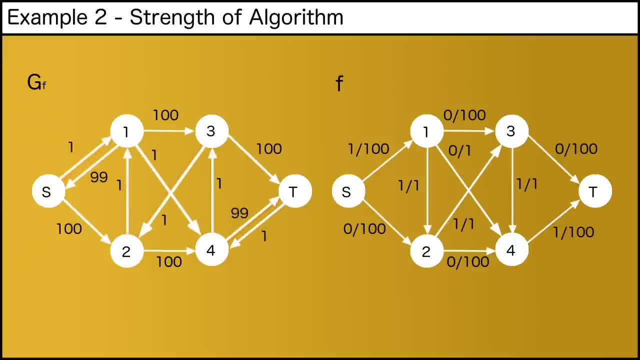 added every time. In this example, you can see that only 1 is being added each time, and this could continue until we find the max flow. Again, by choosing the augmenting path randomly, there is a possibility for a very large runtime. 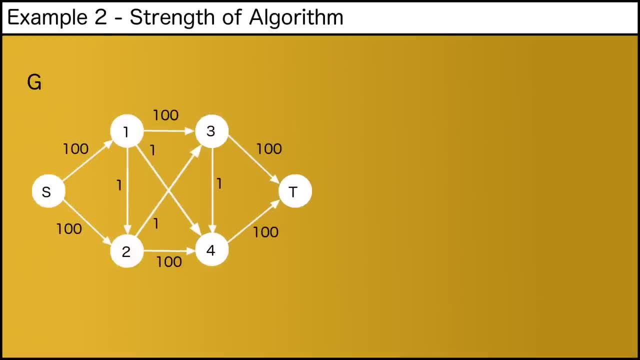 So what happens if we run the Edmonds-Karp algorithm on the same example? In this case it will pick the shortest path each time, going along the top, from s to 1 to 3 to t, and then along the bottom, from s to 2 to 4 to t. 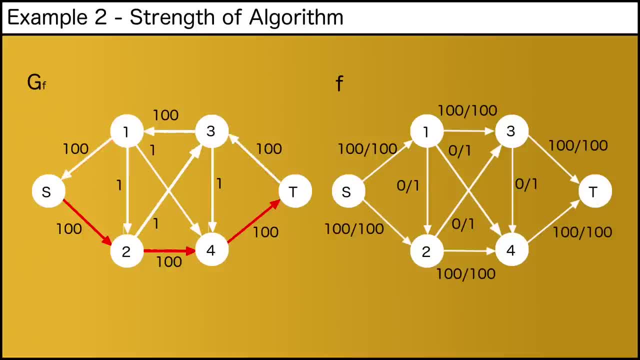 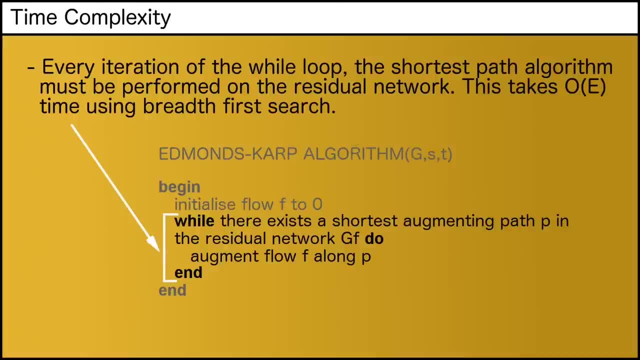 So it will pick the shortest path each time, and then along the bottom, from s to 1 to 3 to t, And then along the bottom, from s to 2 to 4 to t, Or vice versa. the algorithm has terminated in just two iterations of the while loop. 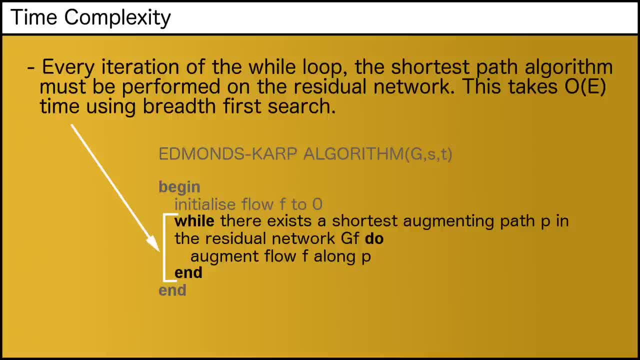 We won't go into the proof, but here is a quick overview of the runtime of the algorithm, Every iteration of the while loop. we have to find the shortest path. This can be done in order of etime using the breadth first search algorithm. So we need to know how many times a while loop can be executed. 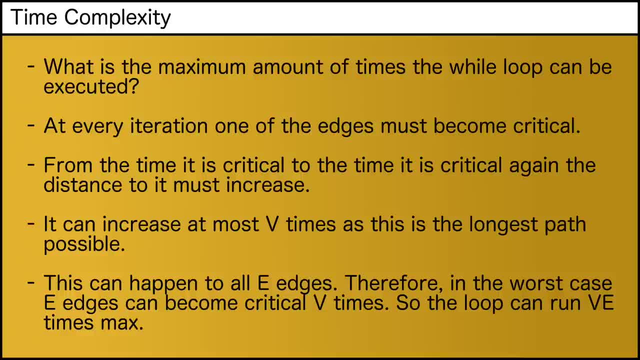 At each iteration, one of the edges has to become critical. So when the time is critical, the path to that edge has to have increased in distance. You might want to pause the video and read over this a couple of times until it sinks in. 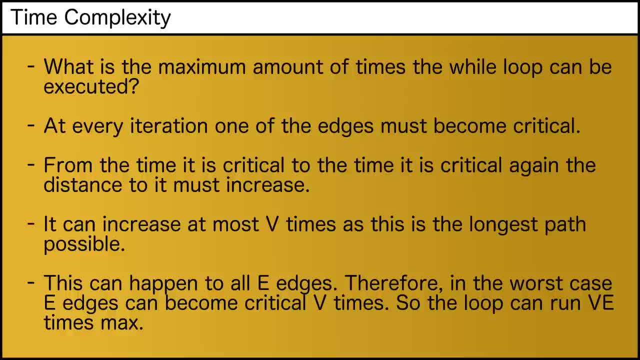 So it can increase at most v times because v is the longest path, a path that goes through every node. In the worst case, this could happen to all e of the edges. So, in summary, all e edges can become critical v times. You can look at the proof for this, but it comes from the fact that we have picked up 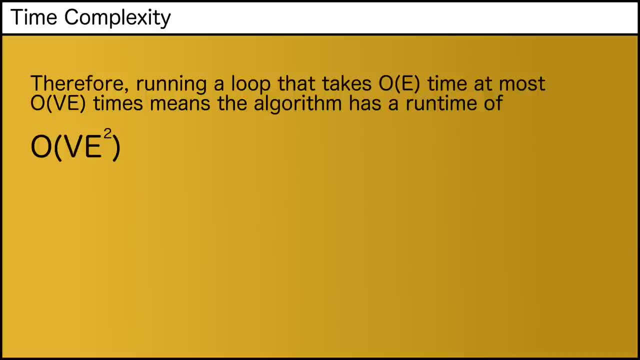 the shortest path. So in the worst case they can be ve iterations and each iteration takes in order of etime. So the overall runtime of the algorithm is in order of v times e squared. Thanks very much for listening. I hope this was helpful. Goodbye, Like comment and subscribe.